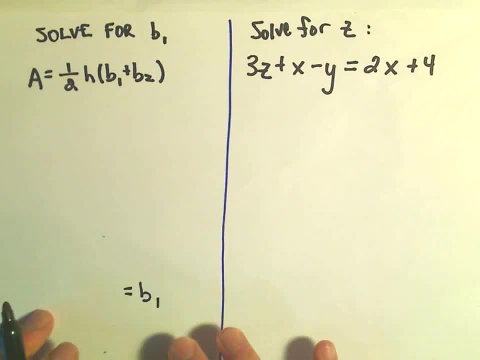 and get b1 all by itself. So there's certainly a couple different ways we can go about doing this. The first thing I notice is that there's a 1 half in here, And typically, if I can get rid of fractions, that's the first thing I like to do. 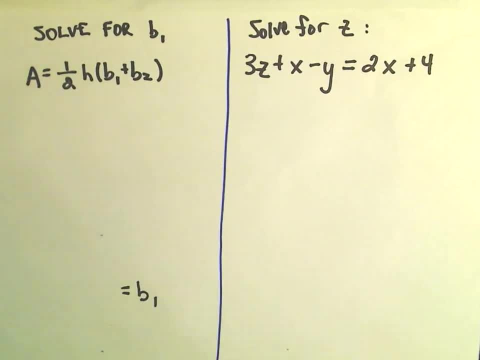 So you know, multiplying by 1, half to me, is the same thing as dividing by 2.. So I think: well, if you're dividing by 2, what undoes multiplication? Or, excuse me, what undoes division? Well, multiplication undoes division. 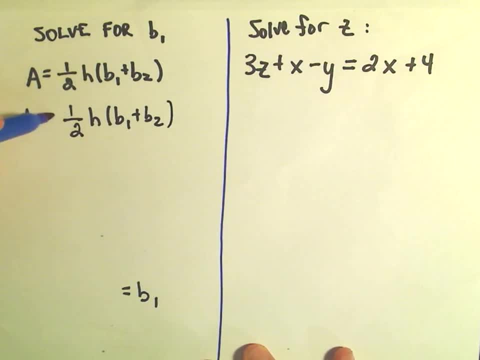 So since we're dividing by 2, to get rid of the 1 half, I could multiply by 2.. But if I do it to the right side, I have to do it to the left side as well. So on the left side we're left with 2a. 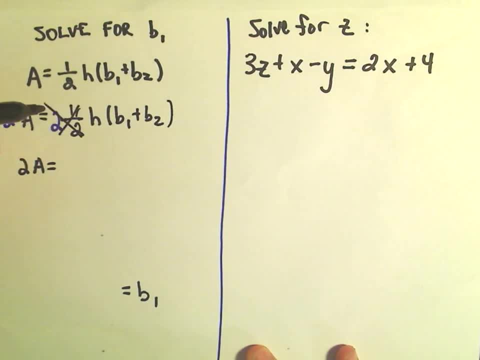 The 2 times 1 half is just 1, so we can basically just get rid of that And then we have h times b1 plus b2.. And now I want to get there's again a couple different ways I could do it. 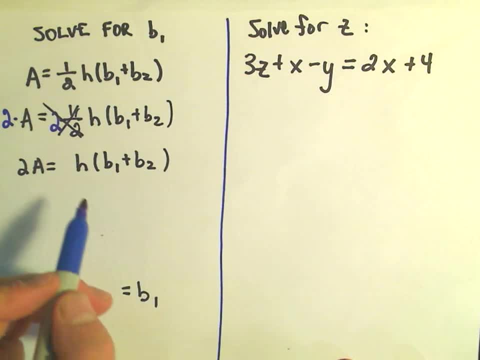 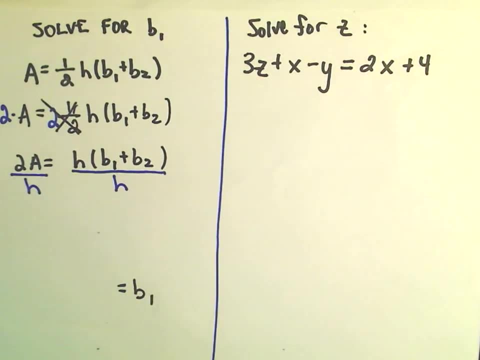 Since I'm multiplying by h, I think, well, I would like to get rid of that. So, again multiplying by h, I'll divide both sides by h. On the right side, h divided by h is just 1.. On the left side, there's really nothing to simplify down, so we still have the 2a over h. 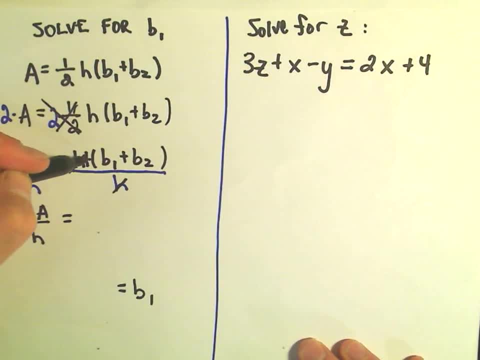 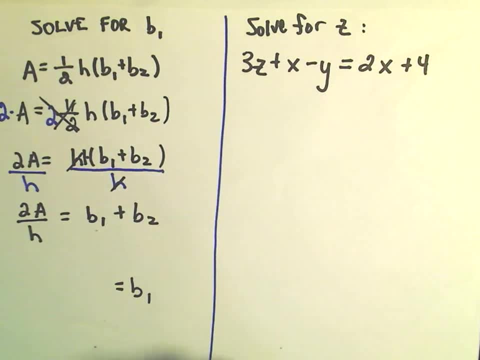 You can think about in the numerator there being a positive 1 in front of the b1 plus b2. If you distribute that, we'll be left with b1 plus b2. And now to simply get b1 all by itself. 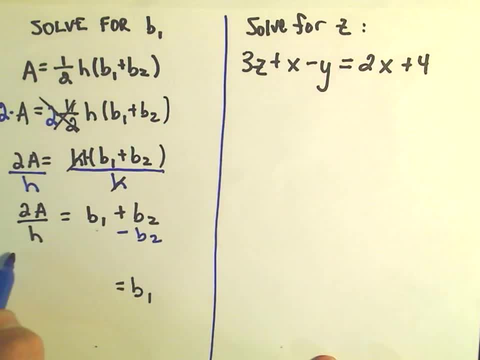 since I'm adding b2, I would subtract b2 from both sides. Well, on the left side we have b1 plus b2. On the right side they're not really like terms, so there's not a lot we can do. 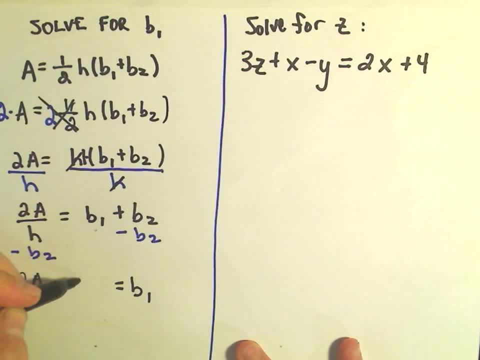 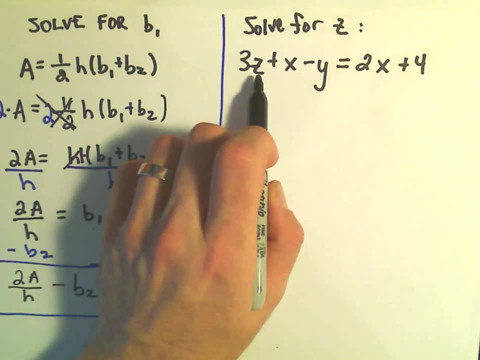 But we do have. we could simply just rewrite it as 2a over h minus b2. And now we have solved for b1. It's all by itself. so we are finished. In the second equation we have to solve for our variable z.